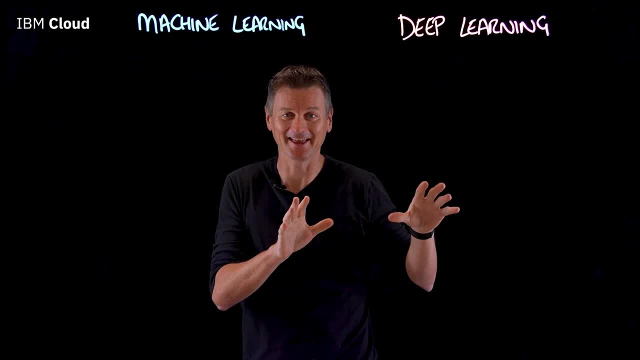 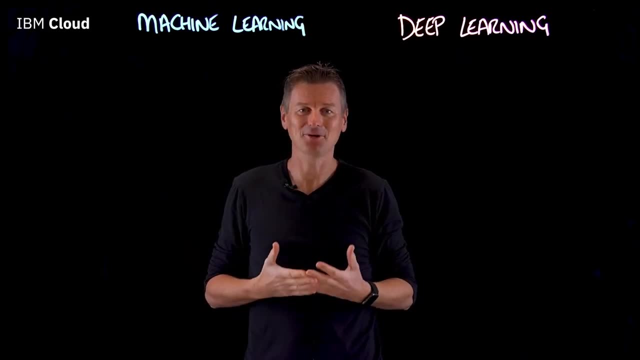 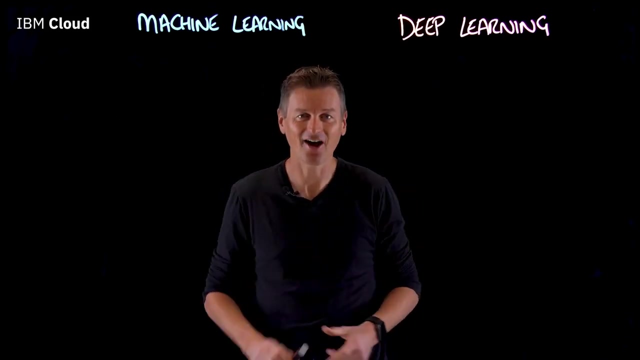 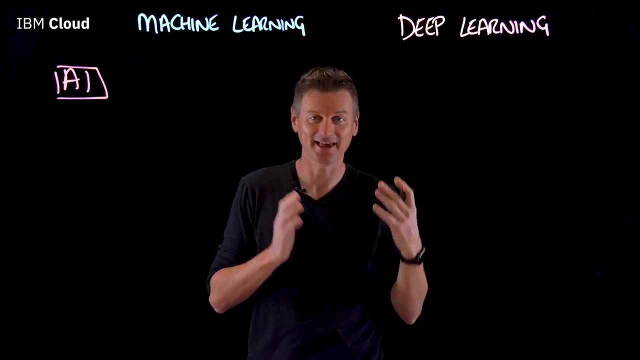 Now, before we get to that, let's address the fundamental question here. What is the difference between these two terms? Well, put simply, deep learning is a subset of machine learning. Actually, the hierarchy goes like this: At the top we have AI or artificial intelligence, Now a subfield. 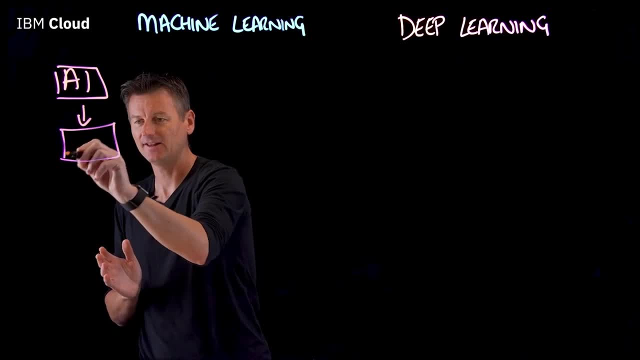 of AI is machine learning, And at the bottom we have AI or artificial intelligence, And at the bottom we have AI or artificial intelligence. And at the bottom we have AI or artificial intelligence, And at the bottom we have ML or machine learning. Beneath that then we have NN. 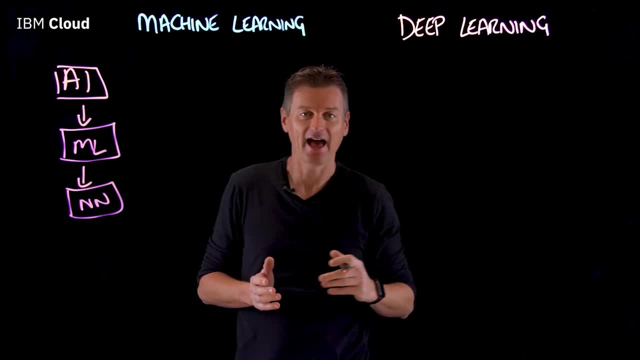 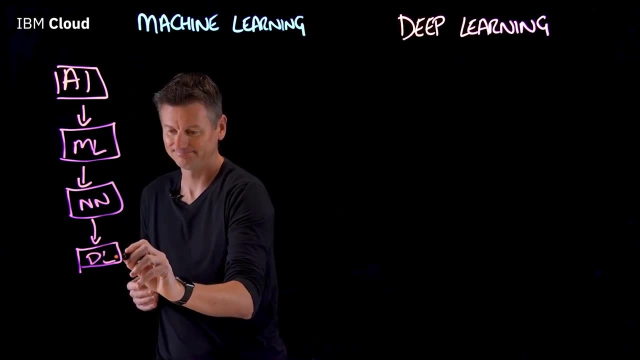 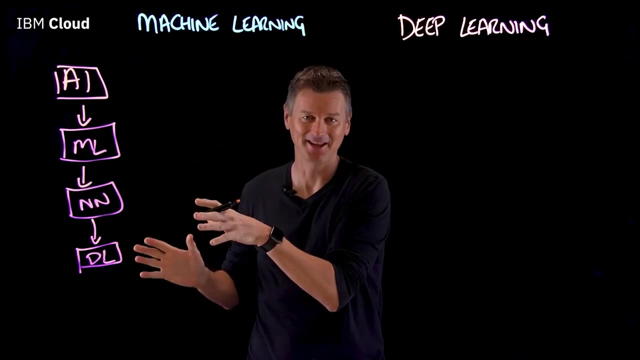 or neural networks, And they make up the backbone of deep learning algorithms, DL, And here on the IBM Technology channel we have a whole bunch of videos on these topics. You might want to consider subscribing Now. machine learning is a subset of deep learning And at the bottom we have AI. 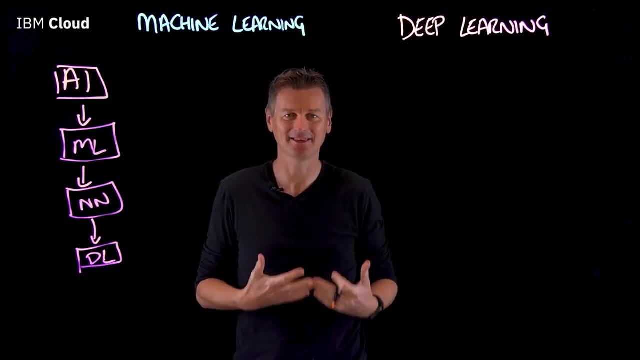 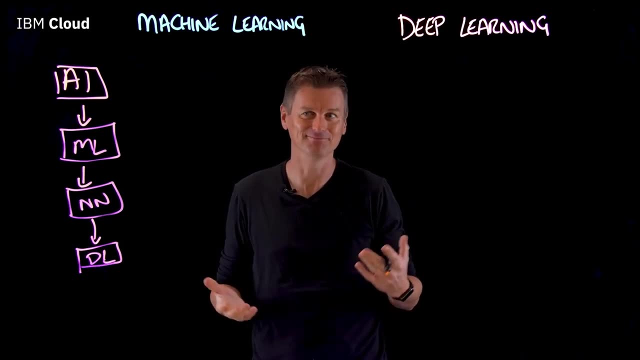 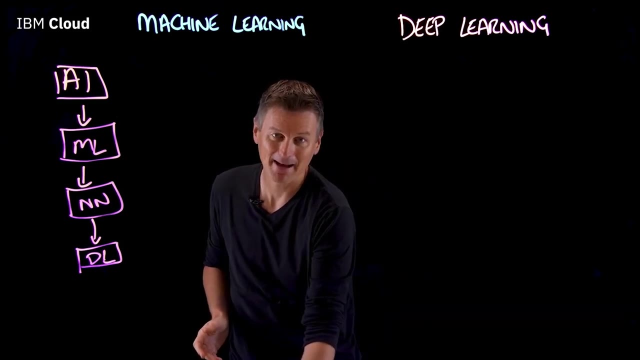 and artificial intelligence. Now, machine learning is a subset of deep learning algorithms, DL, And here on the CORPORATE chain of social defined AI with parallel arrangement. So if I were able to explain to you how you can use a computer to marche through these infrastructures and people, to make predictions, particularly deep learning. 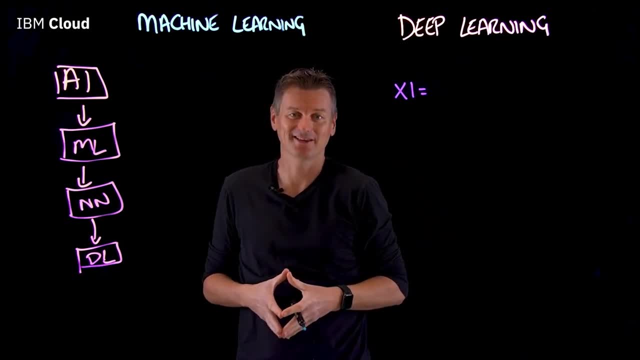 well, I don't want to winter that description, ormouth all yet. Real quickly, I want you to liken it, Shark. We can say yes with a 1 or no with a 0. Yes, it will, so x that equals 1.. 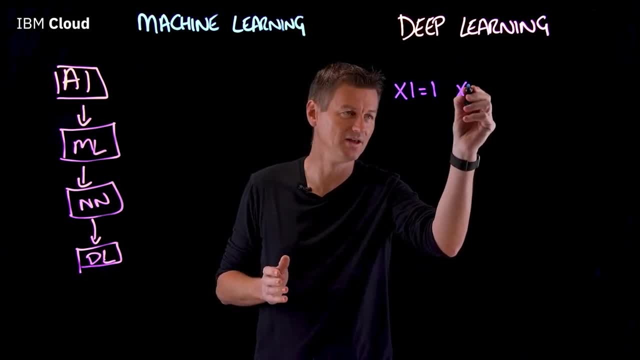 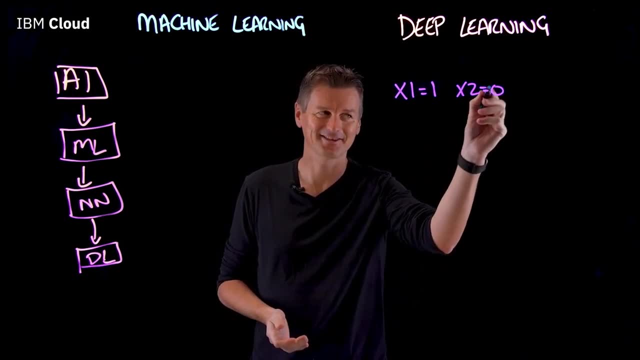 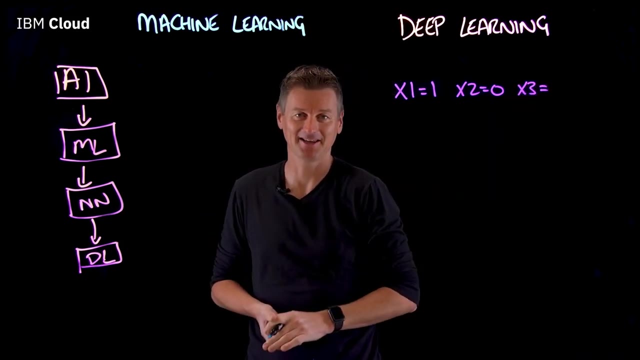 Now x2,. that input says: will I lose weight by ordering pizza? That's a 0,. I'm ordering all the toppings. And x3,: will it save me money? Actually, I have a coupon for a free pizza today, so that's a 1.. 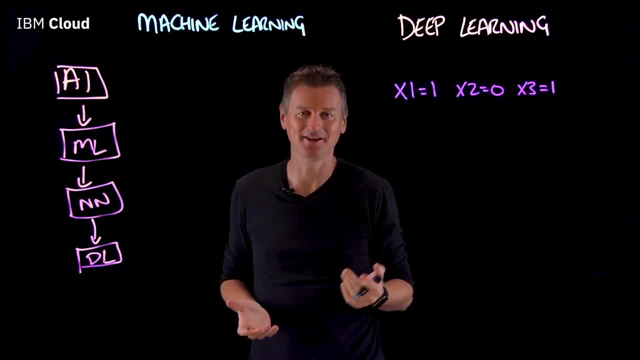 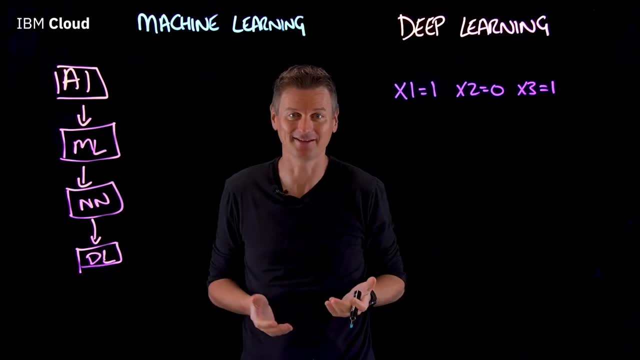 Now look these binary responses 1s and 0s. I'm using them for simplicity, but neurons in a network can represent values from well everything to everything, Negative infinity to positive infinity. With our inputs defined, we can assign weights to determine importance. 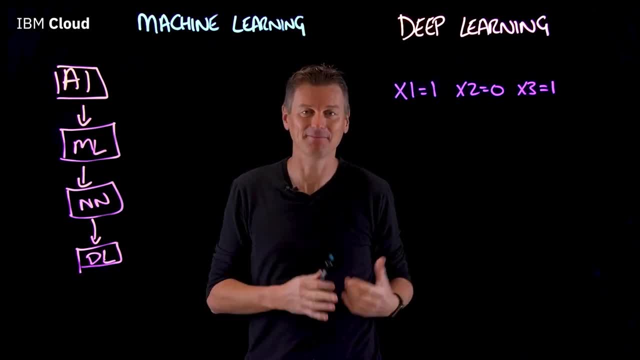 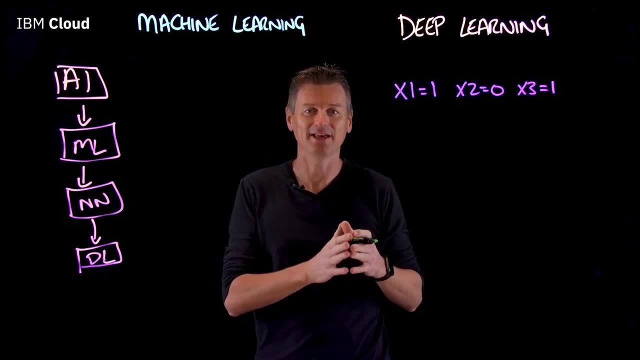 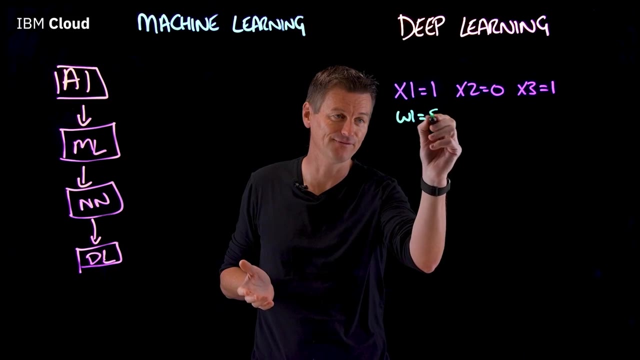 Larger weights make a single inputs contract. That's a contribution to the output more significant compared to other inputs. Now my threshold here is 5.. So let's weight each one of these W1,. well, I'm going to give this a full 5 because I value my time. 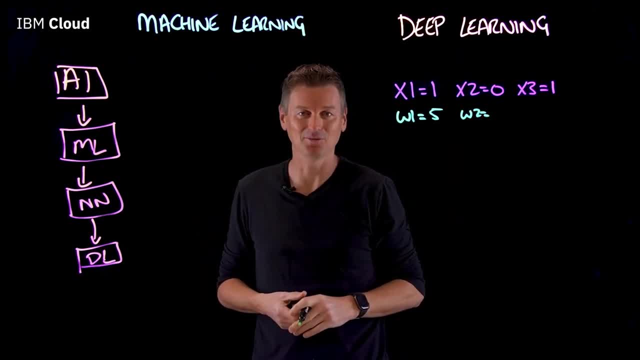 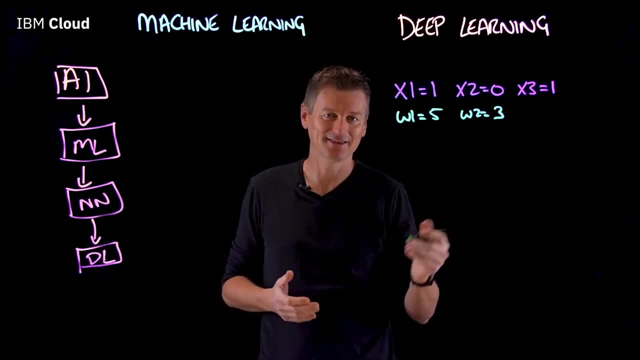 W2, this was the will I lose weight one. I'm going to rate this a 3 because I have some interest in keeping in shape. And for W3, I'm going to give this a 3 because I have some interest in keeping in shape. 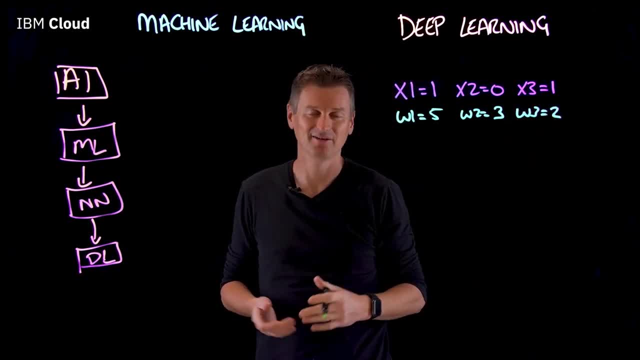 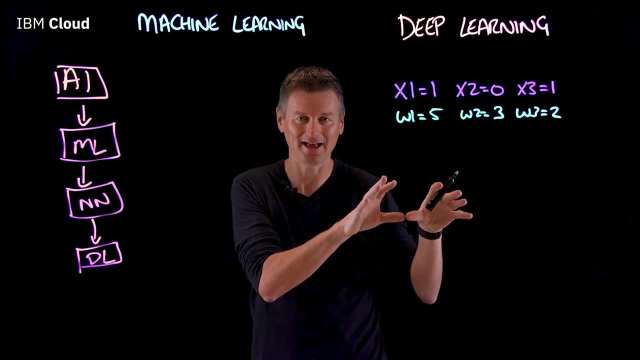 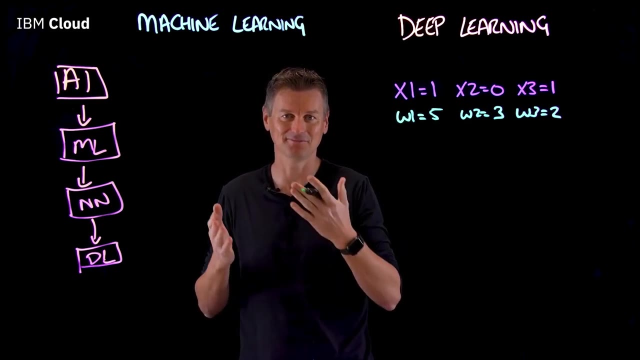 And for W3, I'm going to give this a 2 because either way, this isn't going to break the bank to order dinner. Now we plug these weights into our model and, using an activation function, we can calculate the output, which, in this case, is the decision to order pizza or not. 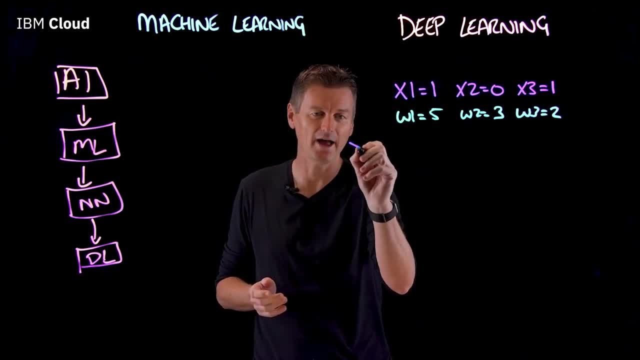 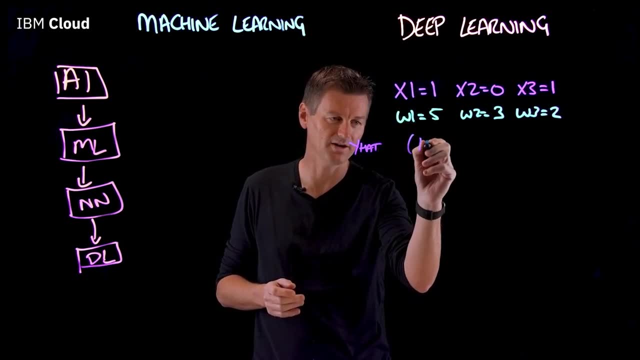 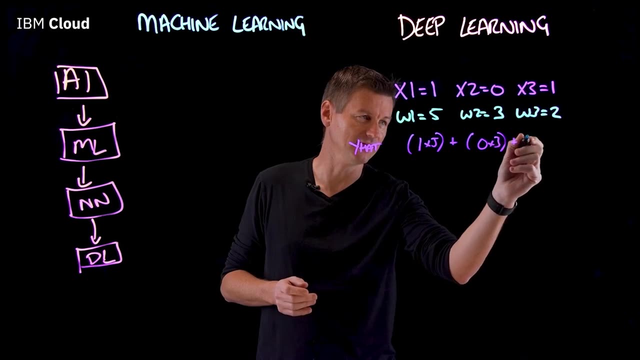 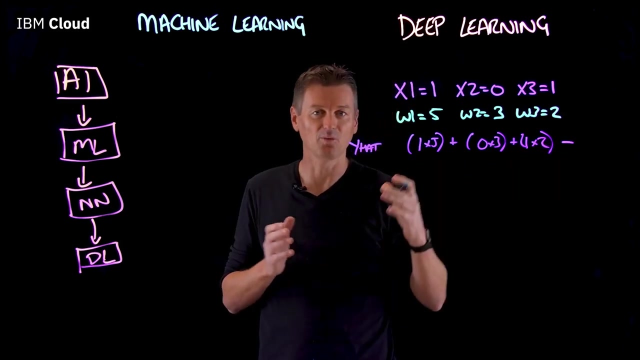 So to calculate that, we're going to calculate the y hat and we're going to use these weights and these inputs. So here we've got one times five, we've got zero times three and we've got one times two, And we need to consider as well our threshold, which was five. 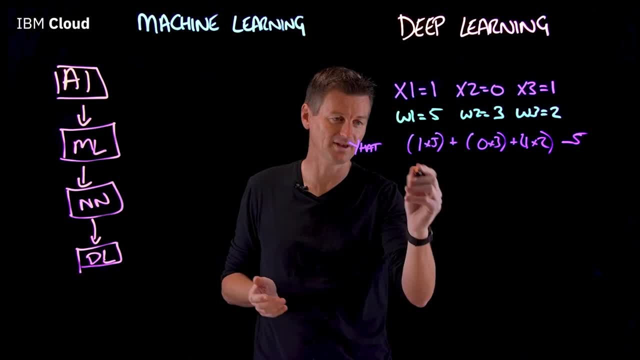 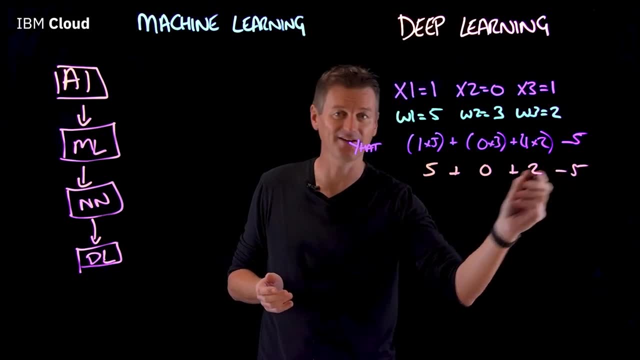 So that gives us, if we just add these up, one times five, that's five plus zero times three, that's zero plus one times two, that's two minus five. well, that gives us a total of positive two. 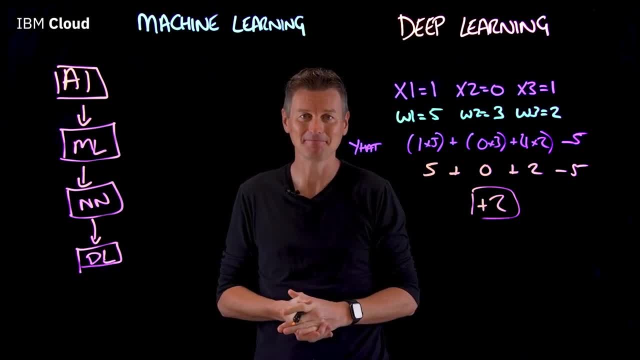 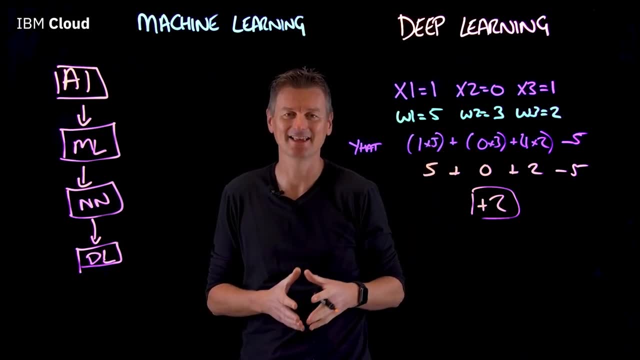 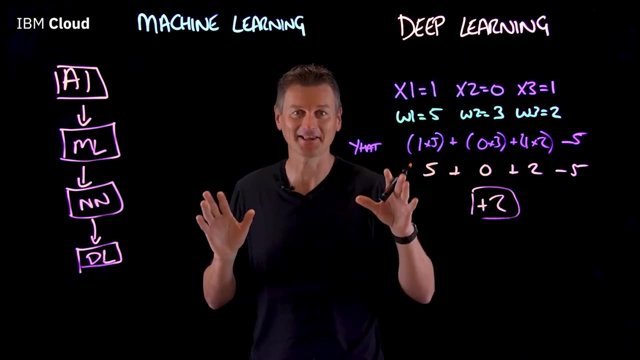 And because the output is a positive number, this correlates to pizza night. Okay, so that's machine learning. But what differentiates deep learning? Well, the answer to that is more than three. As in Classical network is considered a deep neural network if it consists of more than three. 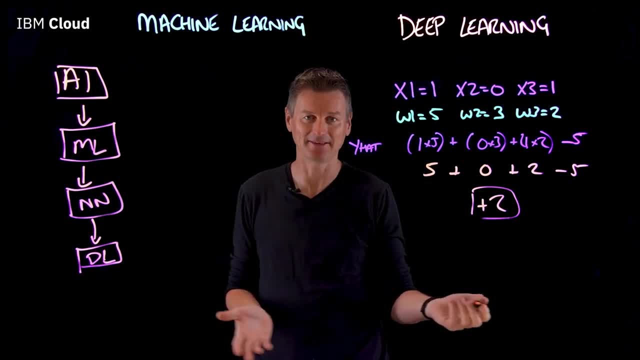 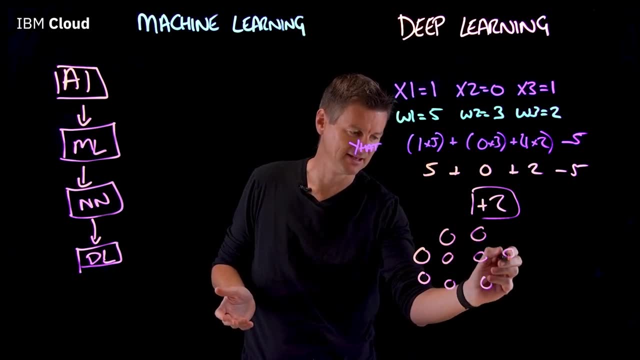 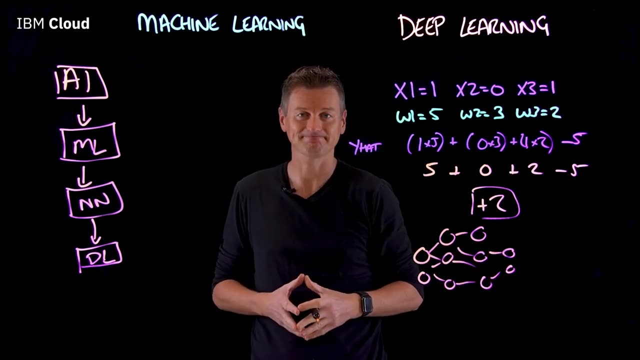 layers, and that includes the input and the output layer. So we've got our input and output. we have multiple layers in the middle and this would be considered a deep learning network. Classical machine learning is more dependent on human intervention to learn. 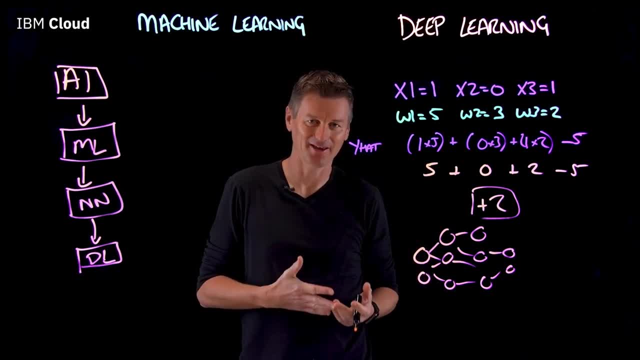 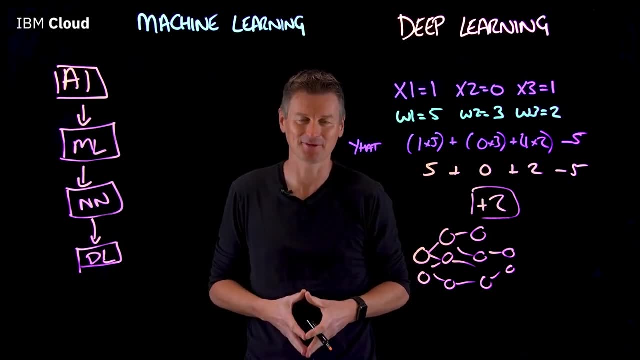 Human experts. well, they determine a hierarchy of features to understand the differences between data inputs. So if I showed you a series of images of different types of fast food, like pizza, burger and taco, you could label these in a data set for processing by the neural network. 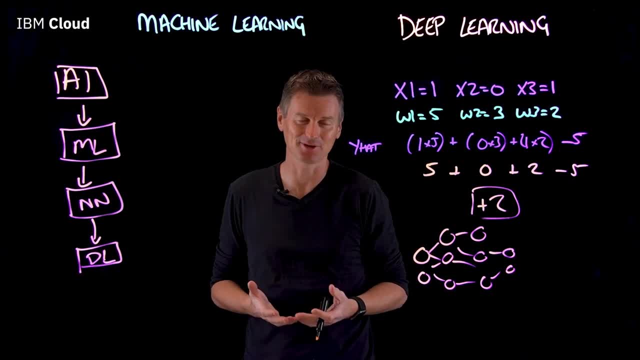 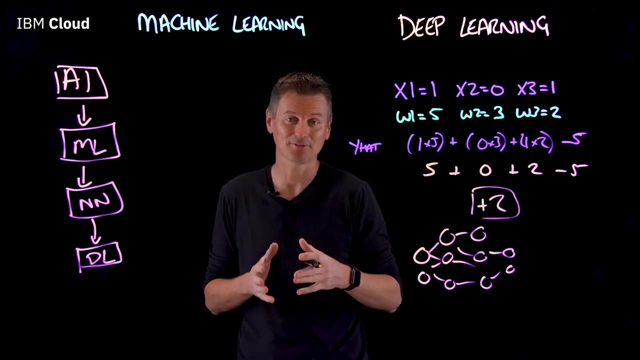 A human expert here has determined the characteristics which distinguish each picture as the specific fast food type. So for example, it might be the bread of each food. That food type might be a distinguishing feature across each picture. Now this is known as supervised learning, because the process incorporates human intervention. 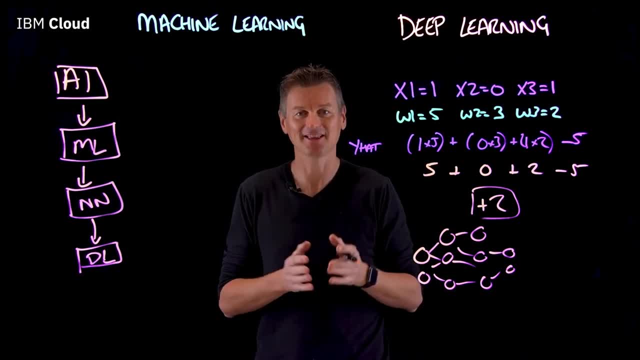 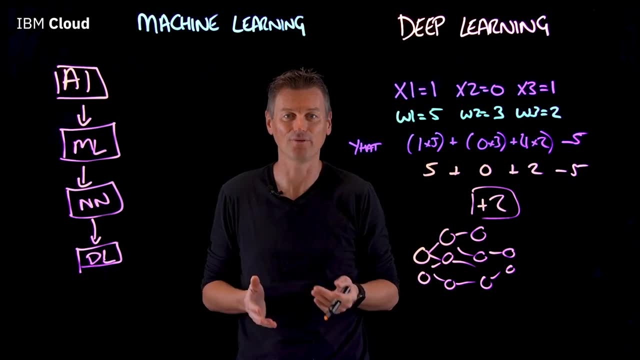 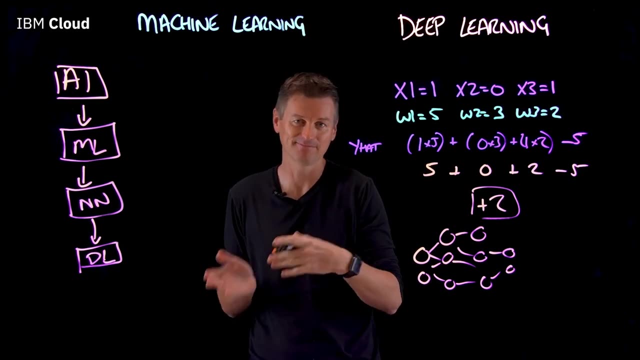 or human supervision. Deep machine learning doesn't necessarily require a labeled data set. It can ingest unstructured data in its raw form, like text and images, and it can automatically determine the set of features which distinguish pizza, burger and taco from one another. 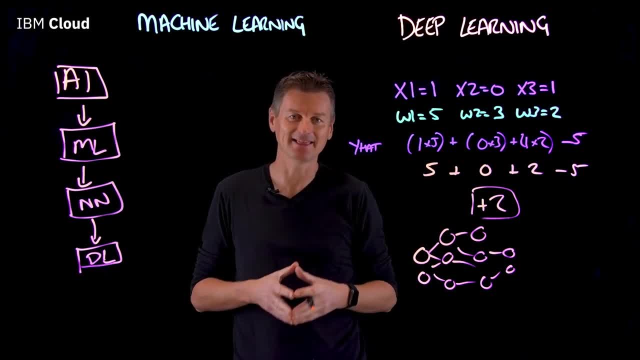 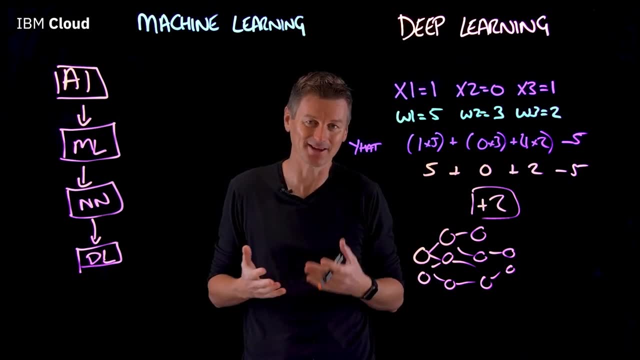 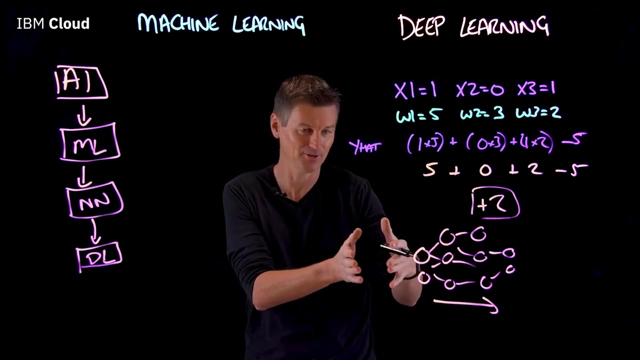 By observing patterns in the data, a deep learning model can cluster inputs appropriately. These algorithms discover hidden patterns of data groupings without the need for human intervention, and they're known as unsupervised learning. Most deep neural networks are feed forward. That means that they go in one direction from the input to the output. 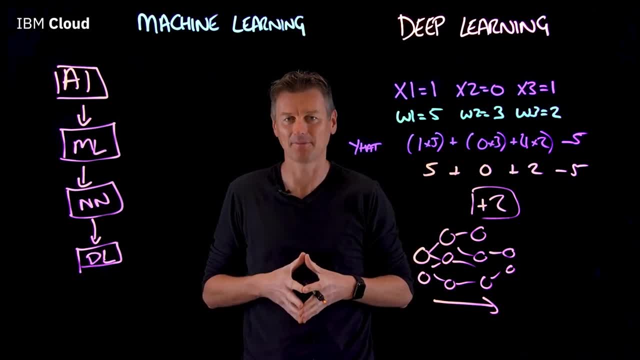 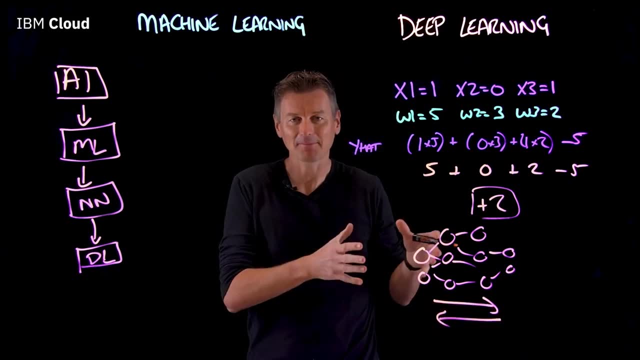 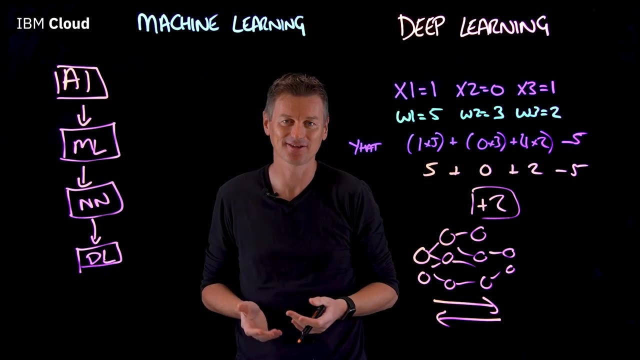 However, you can also train your model through something called back propagation, That is, it moves in the opposite direction from output to input. Back propagation allows us to calculate and attribute the error associated with each neuron and allows us to adjust and fit the algorithm appropriately. 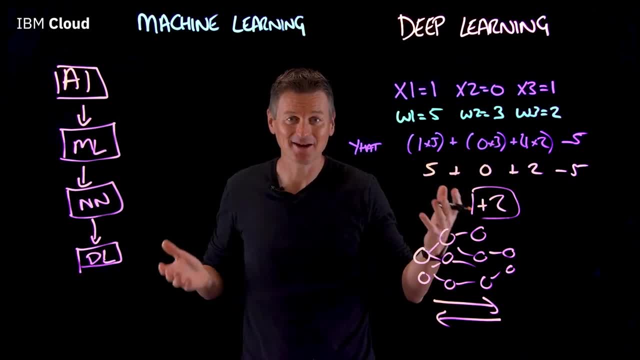 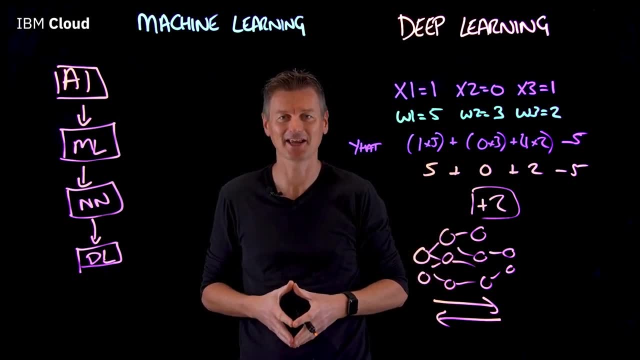 So when we talk about machine learning and deep learning, we're essentially talking about the same field of study: Neural networks. they're the foundation of both types of learning and both are considered subfields of deep learning. The main distinction between the two are that number of layers in a neural network more 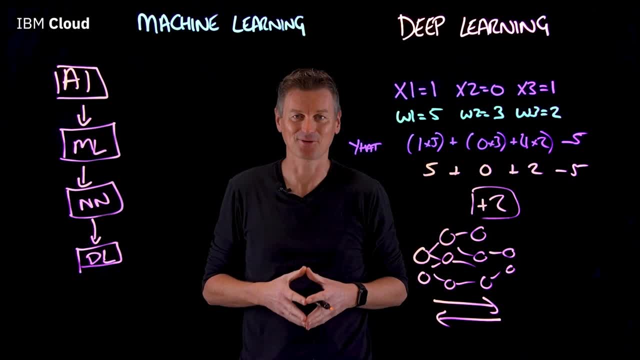 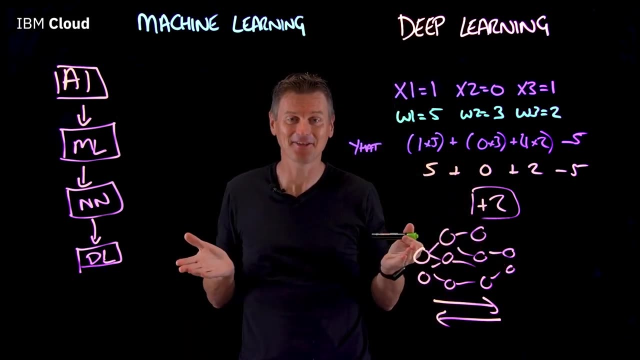 than three, and whether or not human intervention is required to label data: Pizza, burgers, tacos. yeah, that's enough for today. It's time for lunch. Oh, before I go, if you did enjoy this video, here are some others you might also like. 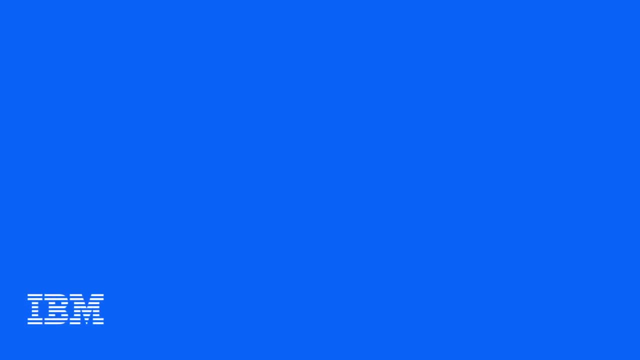 If you have any questions, please drop us a line below, And if you want to see more videos like this in the future, please like and subscribe. Thanks for watching.